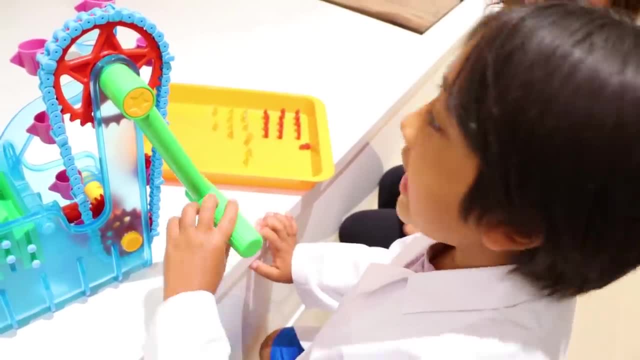 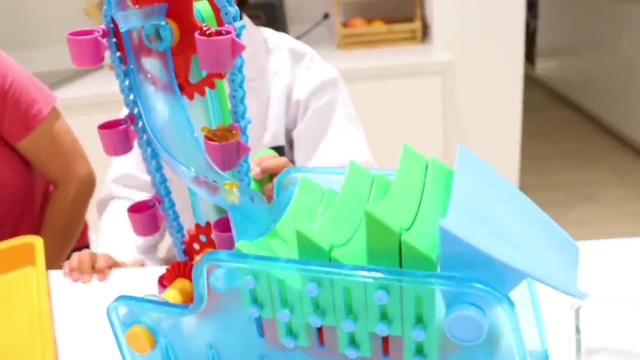 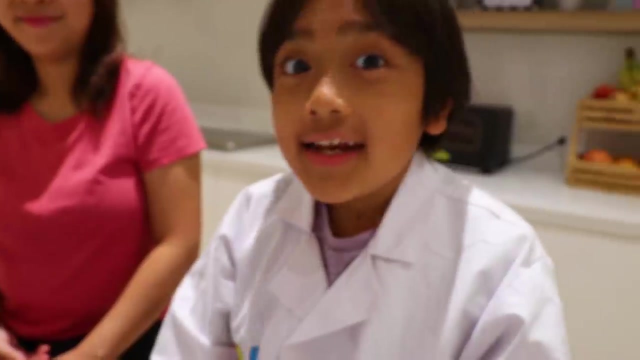 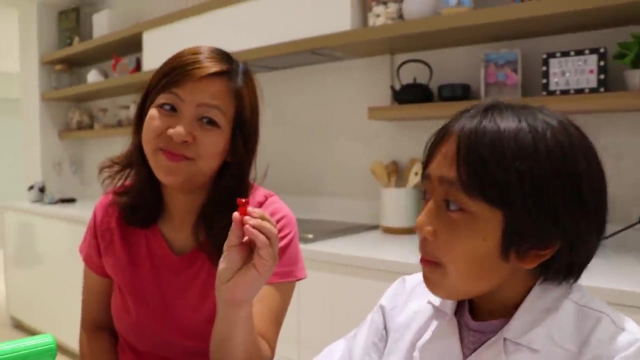 Now we're going to crank the handle. Wooo, Oh Yeah, Wooo. More gummies, Oh Yeah, Now we can enjoy some gummies. All right, combo. Sorry, but you're going into my mouth. 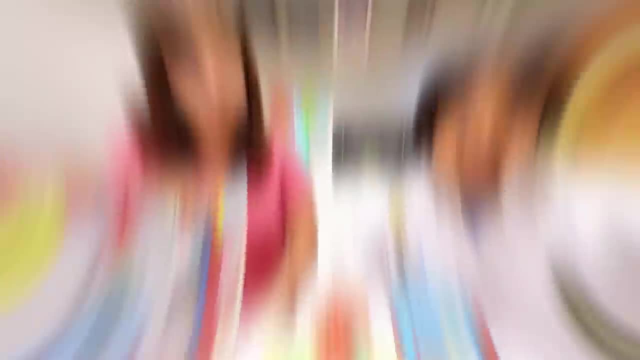 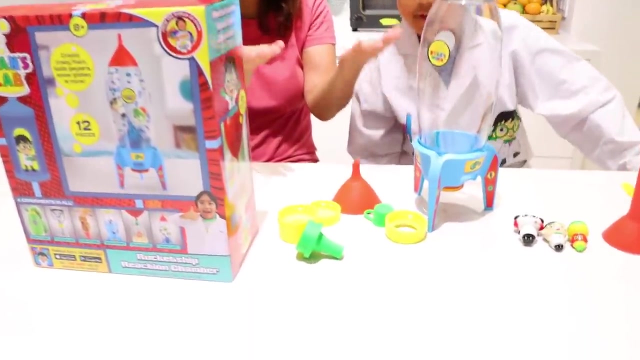 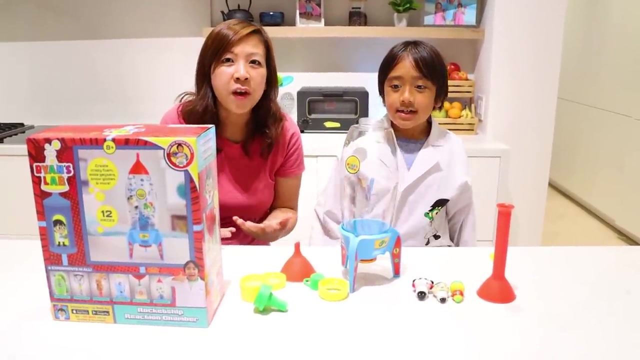 Mmm, Oh, Now we're going to do the Ryan's World Rocket Ship Reaction Chamber. Here's everything that's included for a fun: six experiments. So some of the stuff you do have to get for yourself, For example. first we're going to do one of my favorite, the Soda Geyser. 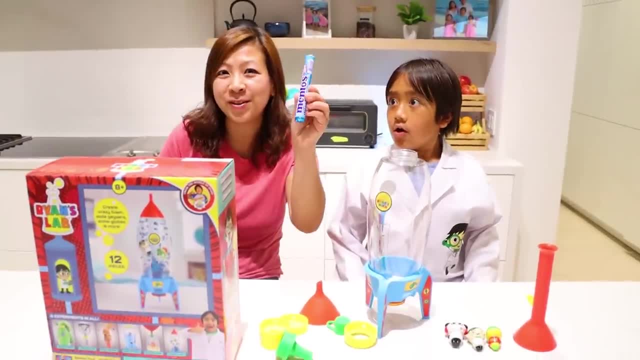 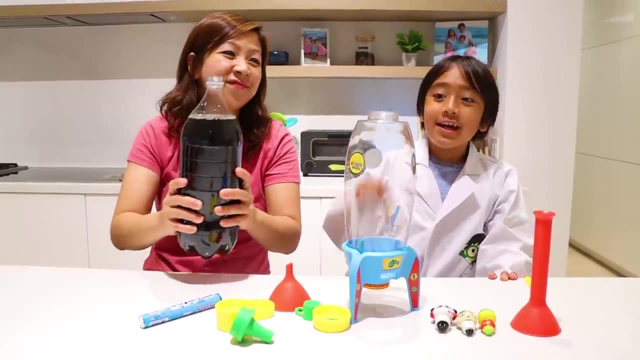 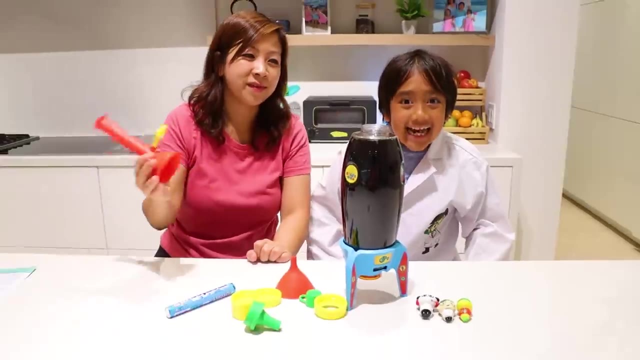 So that means you have to buy your own Mentos and carbonated soda. Okay, first Mommy will put the carbonated soda into the rocket. Thank you, All right. Next we're going to screw in the geyser. 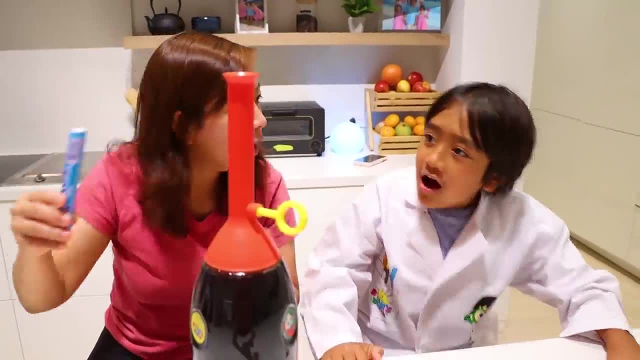 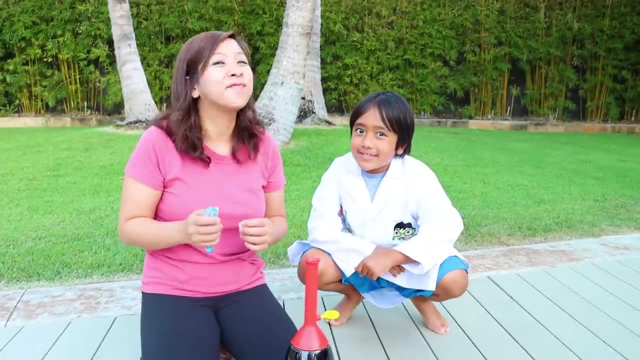 Next put in the Mentos. Wait, This might get a little bit messy. I think we should put it outside. Good idea: Now we're outside, We can add in the Mentos. Okay, add in. Add in. 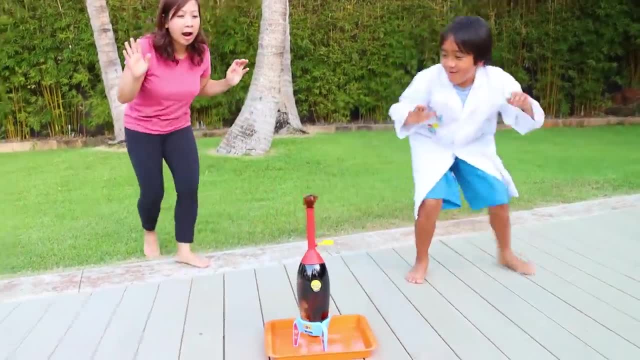 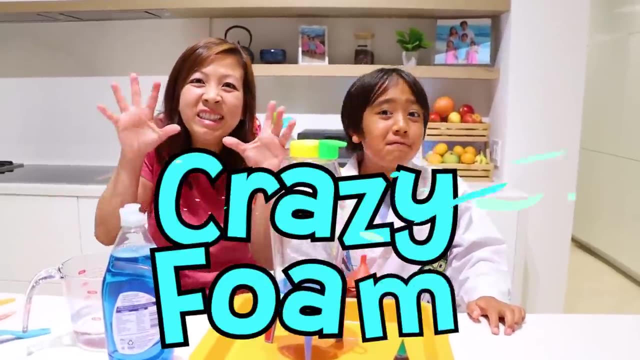 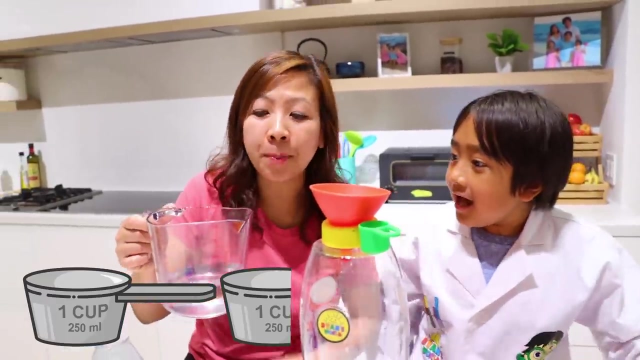 Add in. Okay, now let's pull the pin. Whoa, Whoa, That was so cool. Next is the crazy foam experiment. First you put the funnel on top, Then you can add one and a half cup of hydrogen peroxide, which is not included. 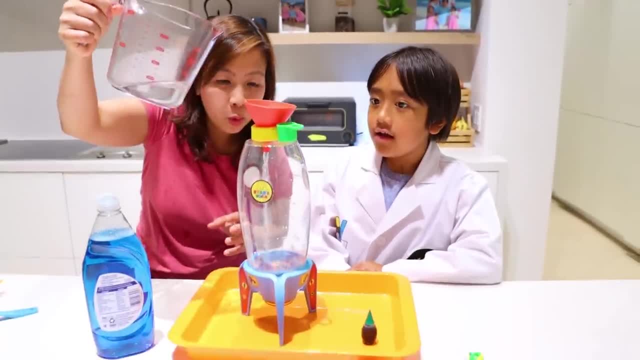 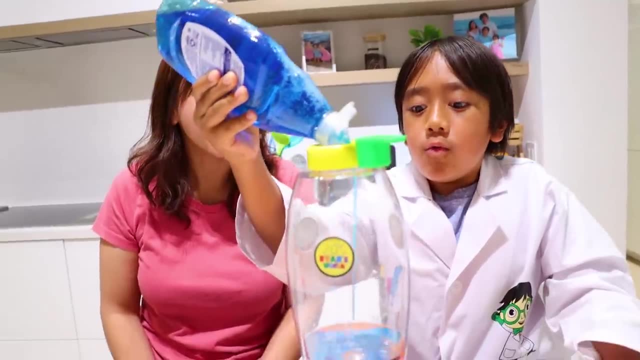 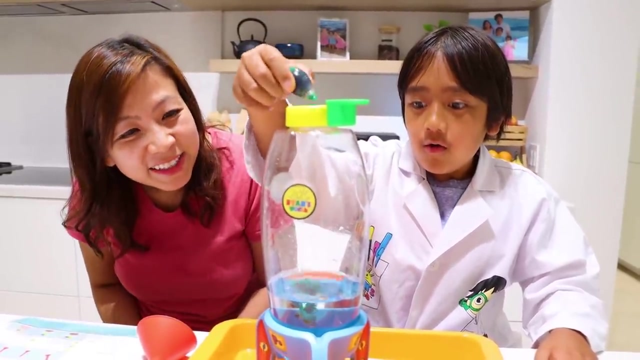 You have to buy it yourself. It's filling up. Next, a big squirt of liquid soap. I'm going to put this in for you. There you go, Okay. Optional, Add some food coloring. I'm doing green. Next, add one tablespoon of dry yeast to three tablespoon of warm water. 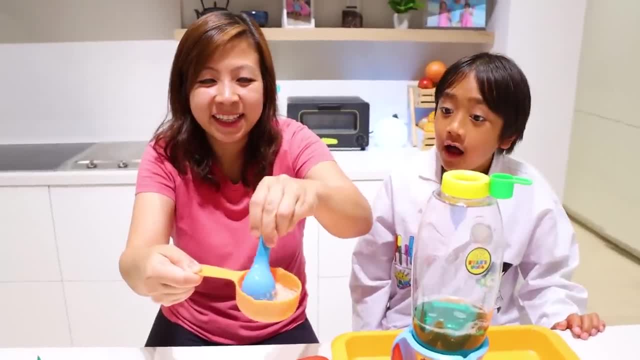 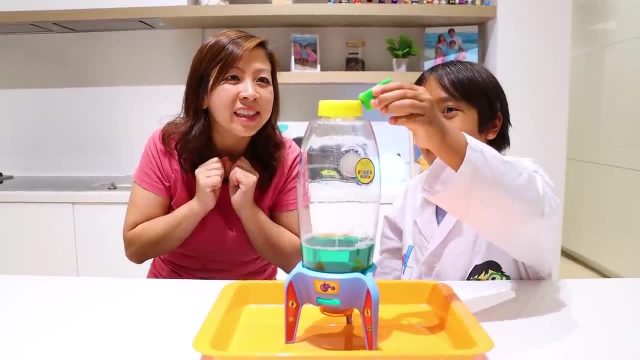 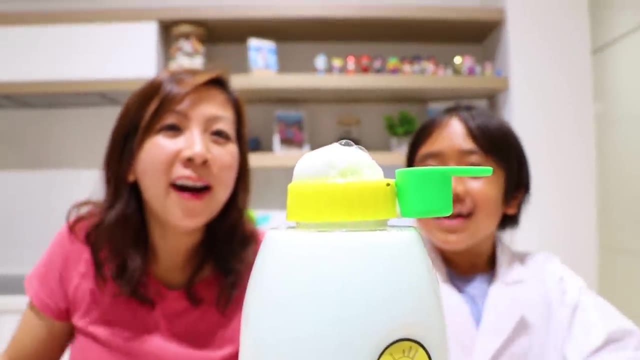 Then stir, Then add it to the attached cup. Now for the foam. Mix it together. Whoooo, Whoooo, Oh. oh it's getting there, Oh it's going in, Whoa, It's exploding. 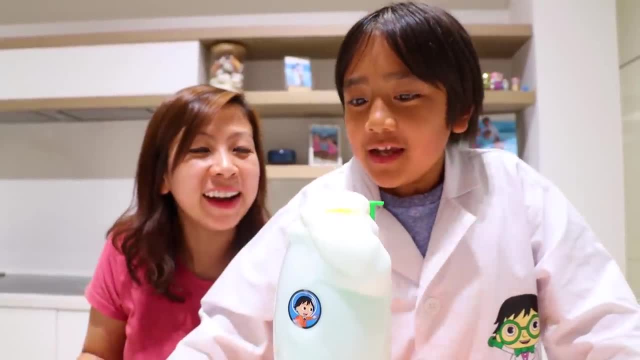 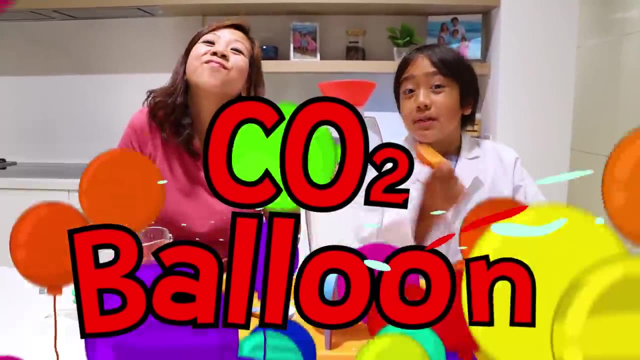 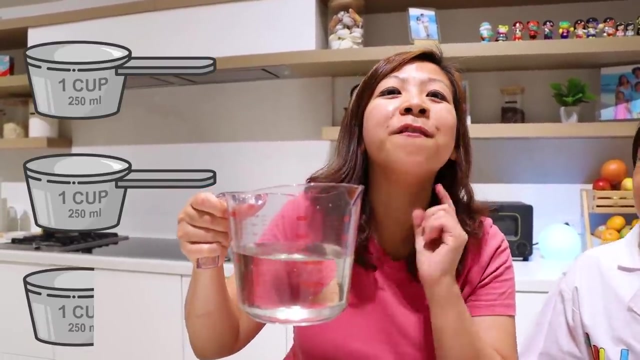 Whoa, They just keep coming. Yeah, Oh, it's coming out. Next experiment is the CO2 balloon. We're gonna blow up this balloon using the rocket ship. First, you're gonna need to get your own two and a half cup of vinegar. 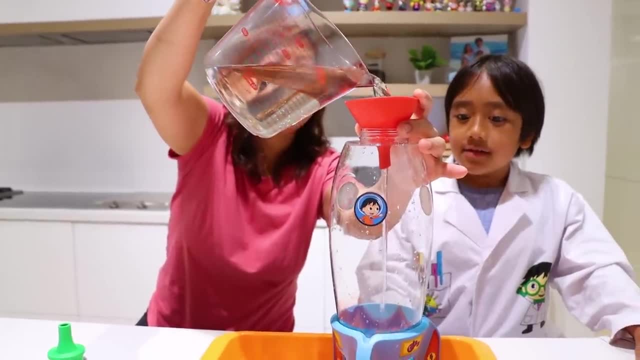 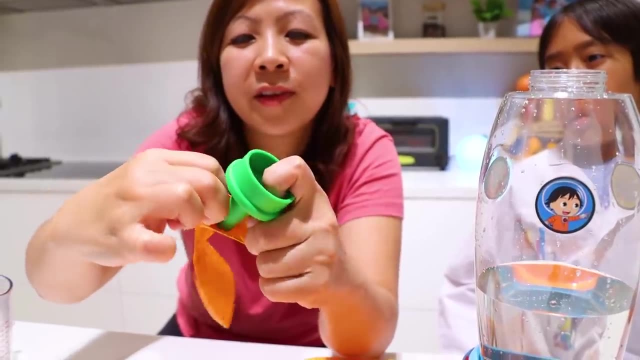 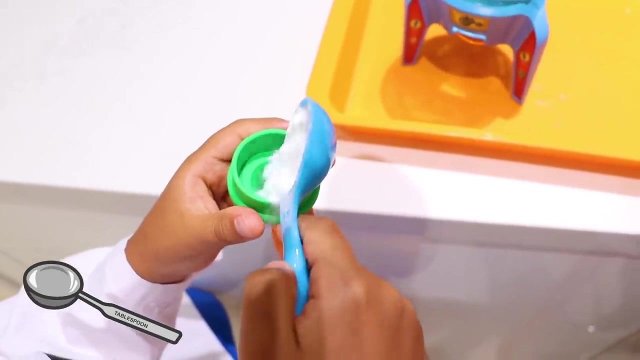 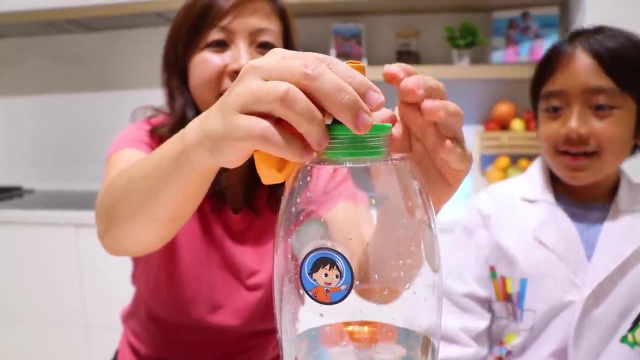 Put it into the rocket carefully. Next, stretch the balloon over the balloon attachment like this. Next, put in one tablespoon of baking soda. Then attach it to the top of your rocket. Plug it in Now. let's mix the baking soda and vinegar. 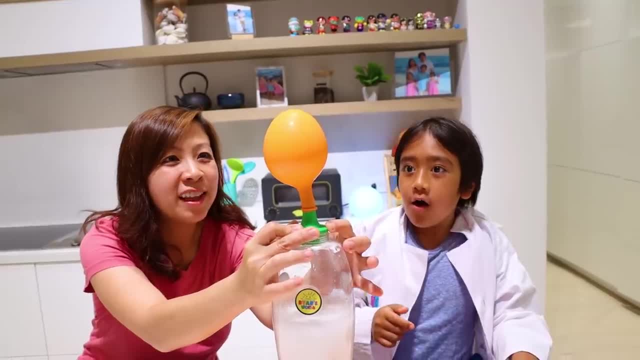 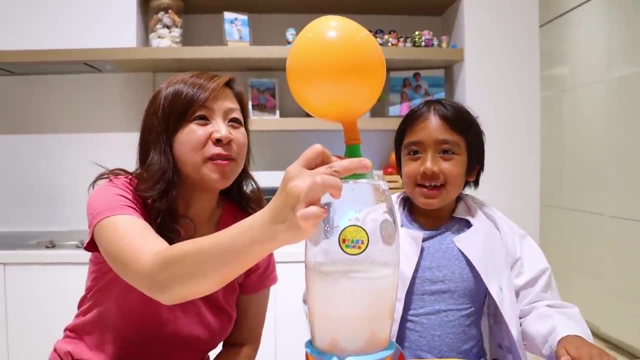 Whoa, look The balloon. Yeah, it's filling. We blew up the balloon using CO2, carbon dioxide. Yeah Yeah. Next we're gonna make a tornado in a rocket, That's right. So first you're gonna get your own two liter bottle. 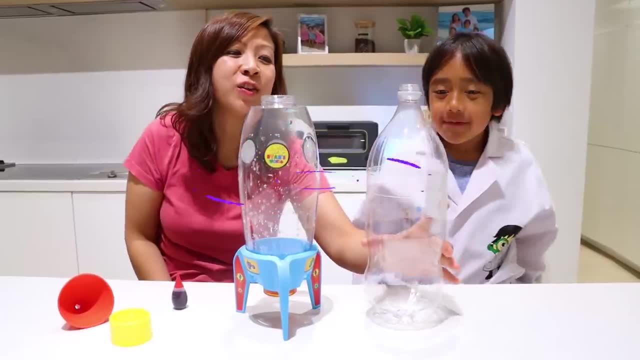 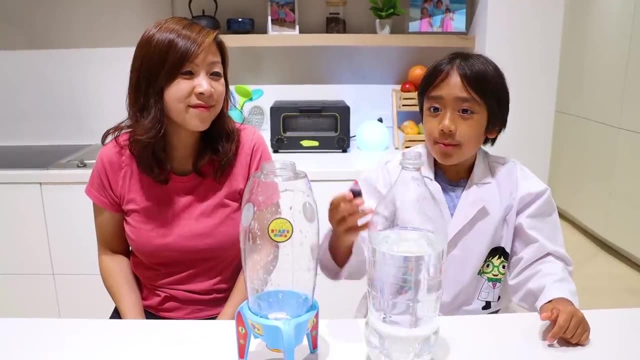 and fill it up with water. Add water. Next, I'm gonna put red food coloring- Optional, of course. Next, screw in their tornados, And then we're gonna put in a little bit of vinegar, And then we're gonna put in a little bit of vinegar. 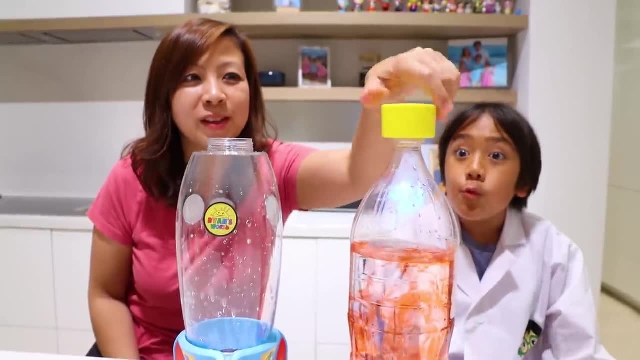 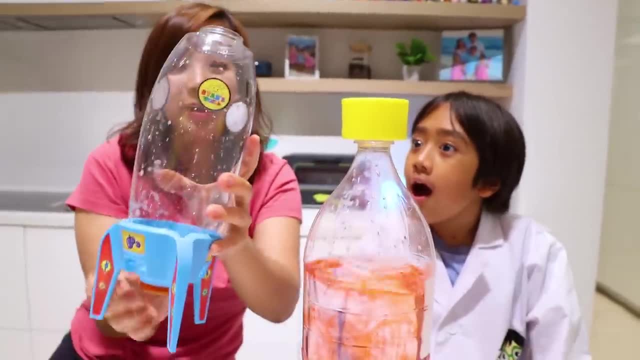 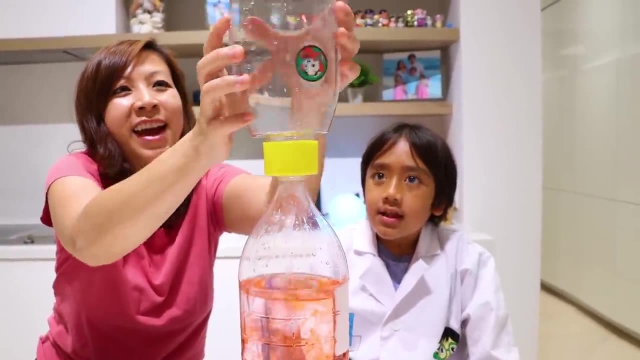 Then, using the rocket, turn it upside down, Ooh, And then twist and turn: Whoa, look how tall it is. Whoa, look how tall it is. Whoa, look how tall it is. Yeah, Are you guys ready to see a super tiny. 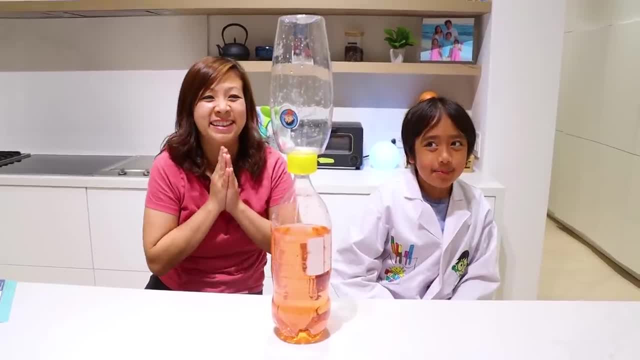 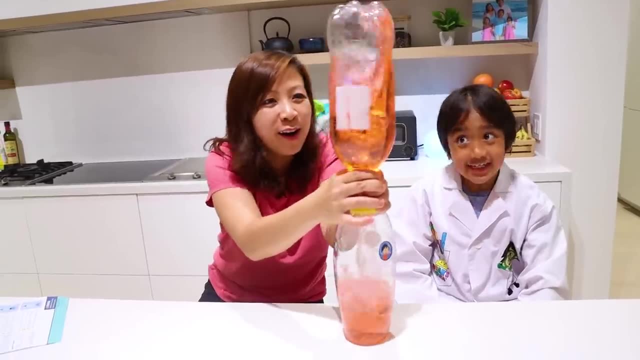 water-nado in real life. Yeah, Take it away. Assistant Mommy. Okay, Now you're gonna flip it upside down while spinning. Whoa, whoa, whoa, whoa- I'm getting dizzy. Whoa. 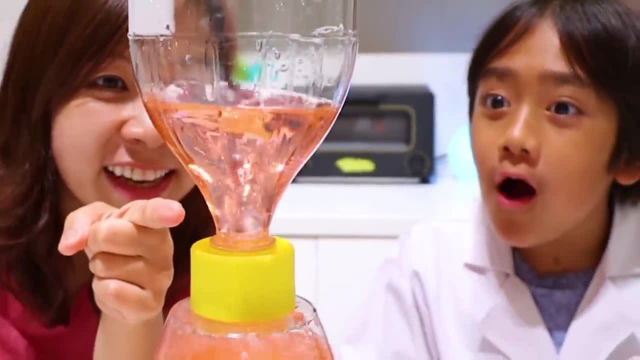 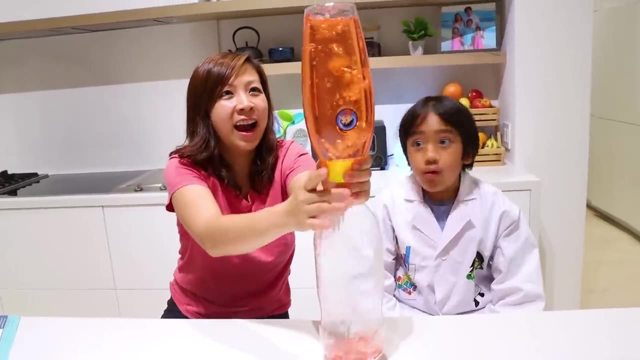 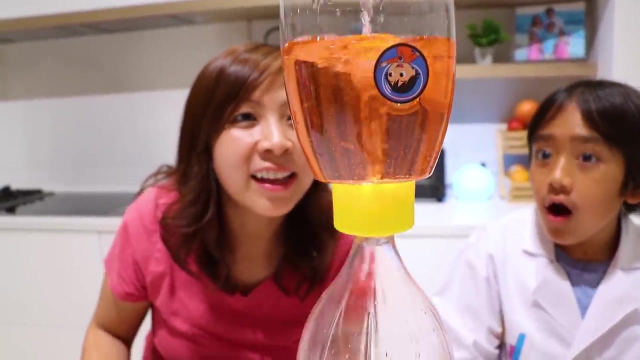 Look, Whoa, Do you see it? Yeah, Then you can just do it again, Turn it upside down, Brr, And then spin, Spin, spin, spin, spin. Whoa, I'm dizzy. Look, Look at the tornado. 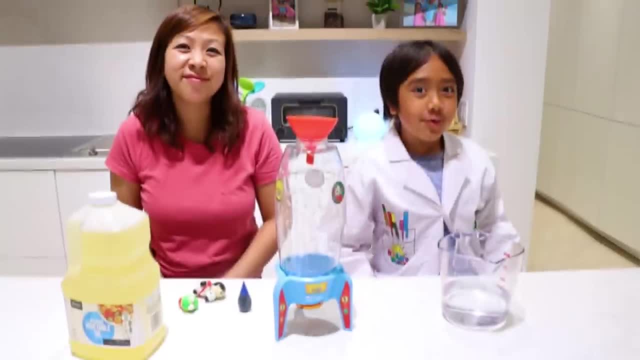 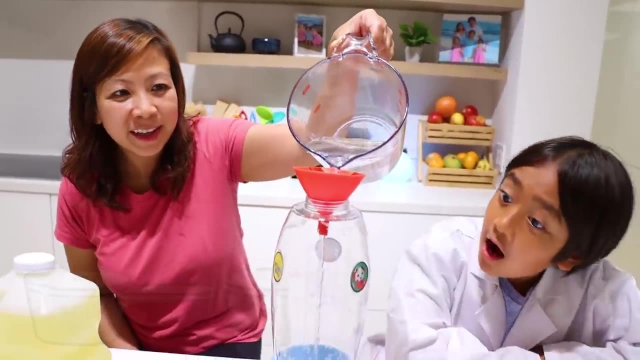 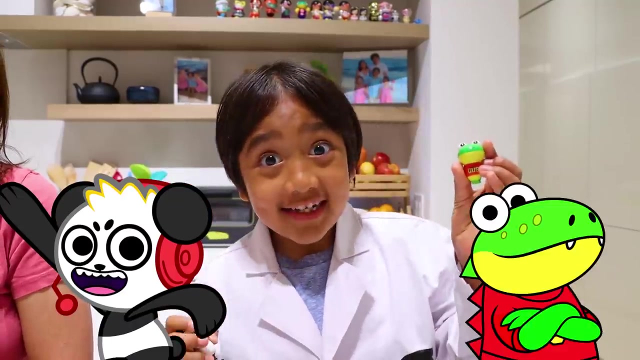 Whoa, Next room space lava experiment. First there's gonna be one and a half cup of water. Next is my favorite part: I'm gonna add some Ryan's World characters like Combo or Gus, or even me, Scientist Ryan. 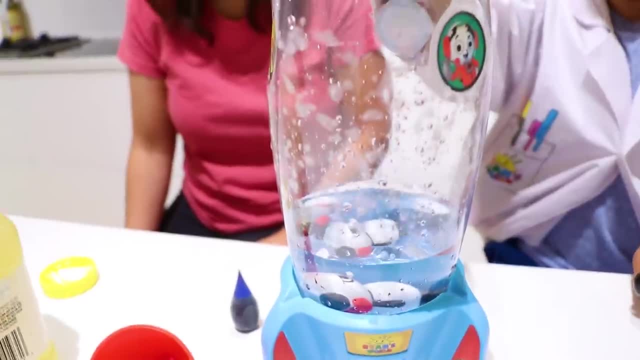 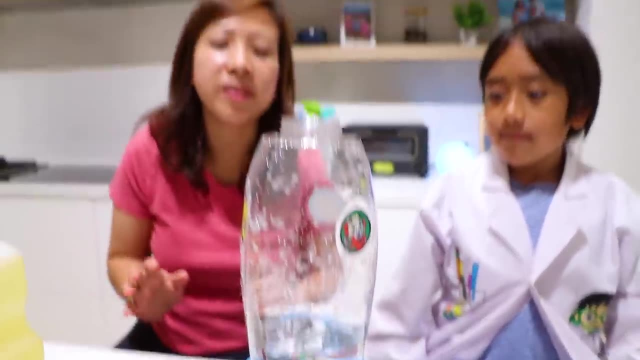 Okay, I'll put Combo in first. Ooh And Gus will go to me, Boink And Scientist Ryan, that's me Fall. So, Ryan, did you notice that they sink or float? They sink, That's right, Ryan. 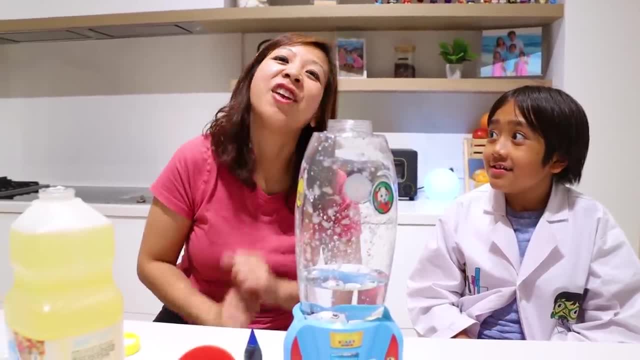 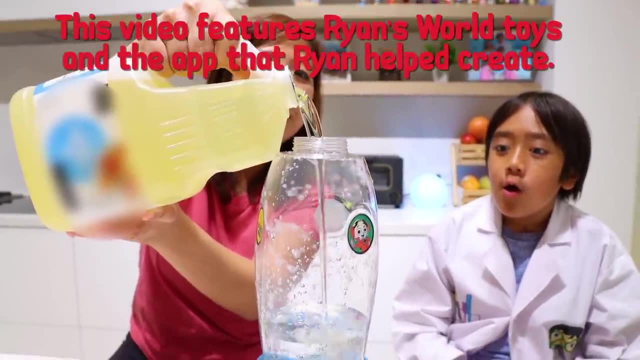 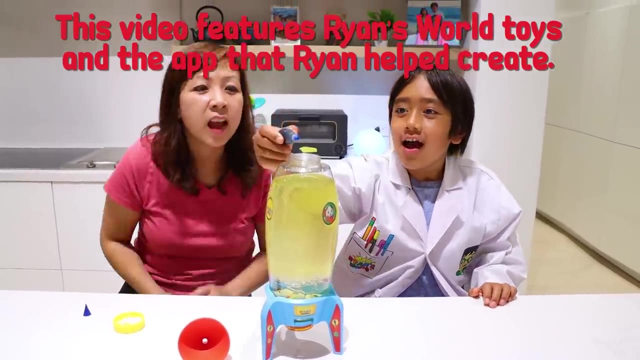 They all sunk. That's because their density is higher than water. Ooh. Step two: using vegetable oil, fill it up all the way to the top, Whoa. Next, add 10 drops of food coloring. One, two, three, four, five, six, seven, eight, nine, 10.. 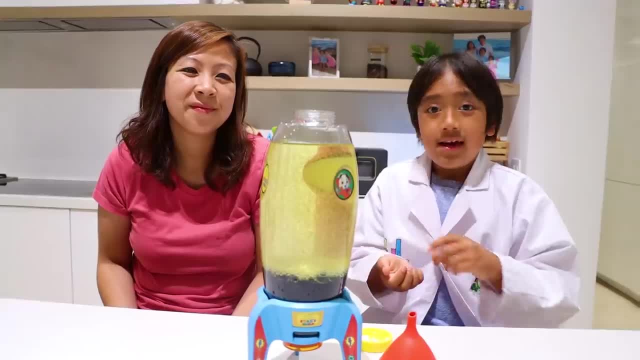 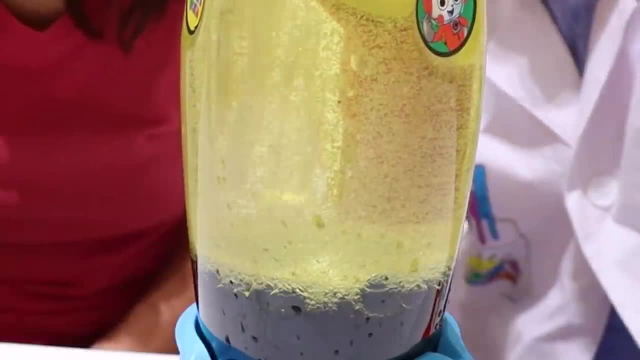 Whoa, Look it's going down. Whoa, Now time to put in the seltzer tablets. I'm gonna split it in half and drop it in Yep, Oh, Oop, Whoa Space lava, Yeah. 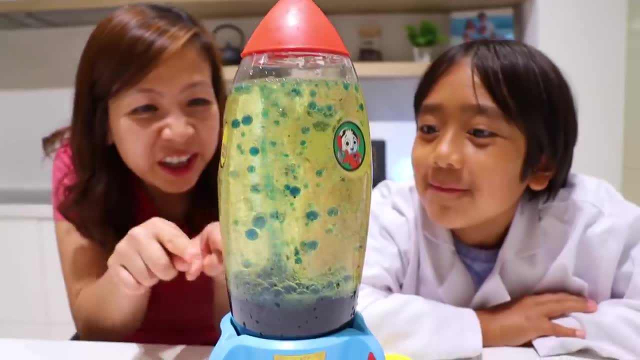 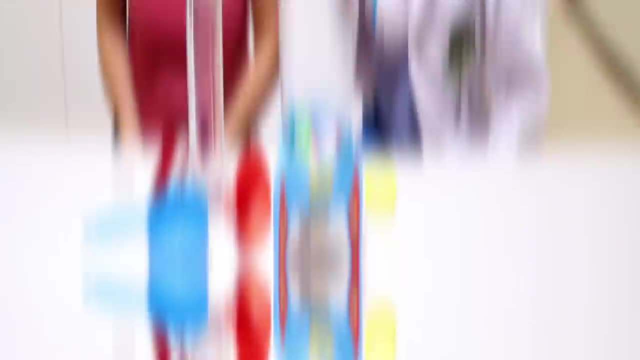 Wait, are the Ryan's World figures gonna go up? I don't know. I think they're in water. Yeah, Woo-hoo, Ooh, Whoa. that looks so cool. Next we're gonna make a snowstorm in a rocket. 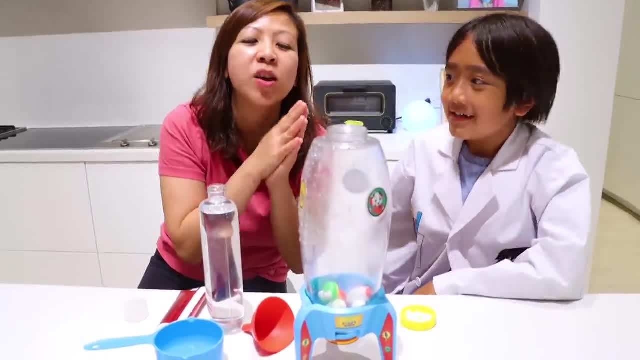 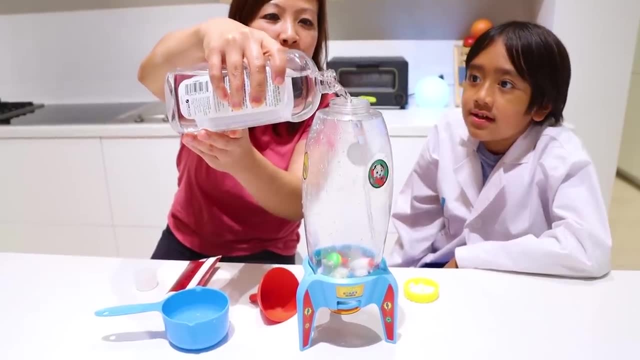 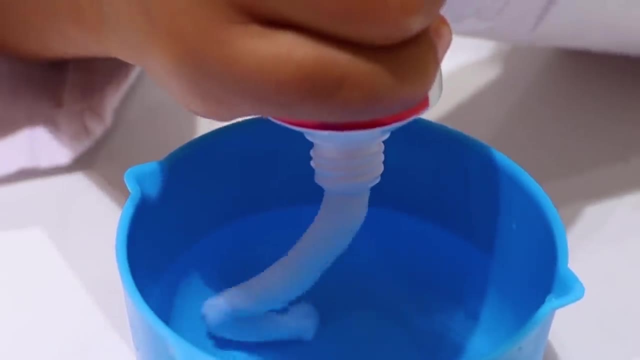 Ah, Just kidding, we're making a snowstorm in here. So first you're gonna do is fill up your rocket with three-fourths full of baby oil- Whoa. Next, add white toothpaste to water. Now we agitate or mix. 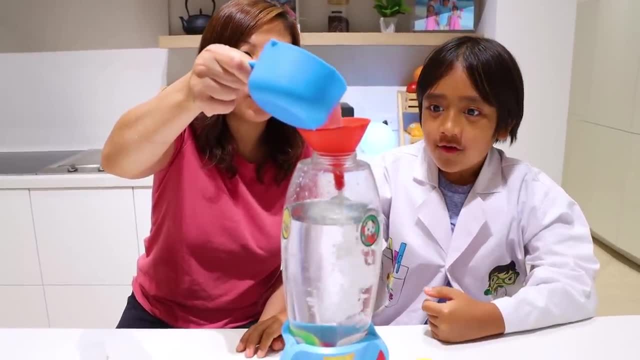 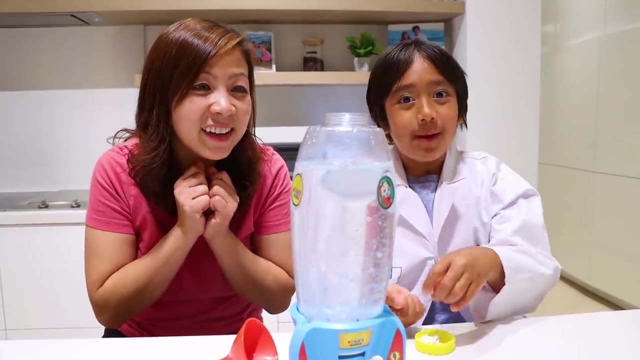 Then you're gonna add the toothpaste and water mixture to the rocket tank. Whoa, Now time to put in the seltzer tablets And then make the snowstorm by putting it in: Boop, boop, boop, boop, boop, boop. 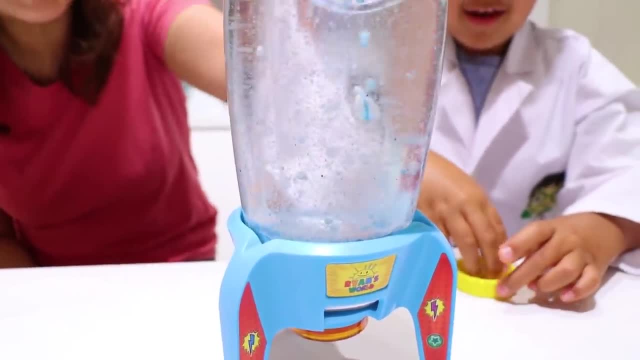 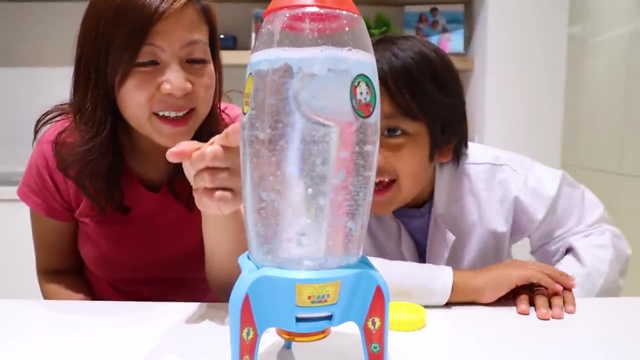 Oh, it's starting. Look it's starting. Yeah, close the cap. Okay, It's a snowstorm. Whoa See, the bubbles keep rising. Oh yeah, Rise and then fall. Cool, Okay, guys. so now we're gonna show you. 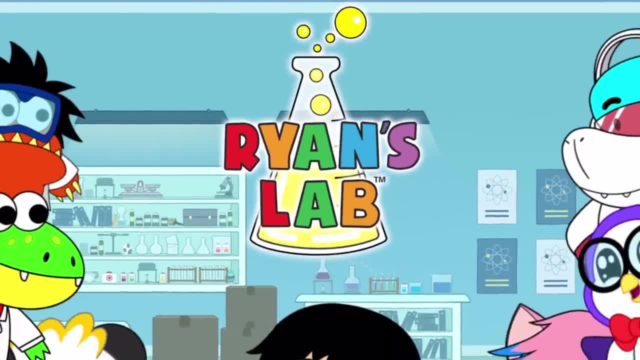 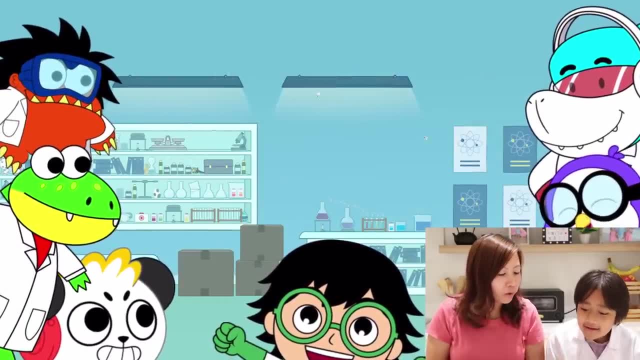 a really fun edutainment app. It's called Ryan's Lab. Let's launch it up here. You see Ryan there with the whole crew. Yeah, So you can have multiple counts. So this is Ryan, obviously. Yeah. 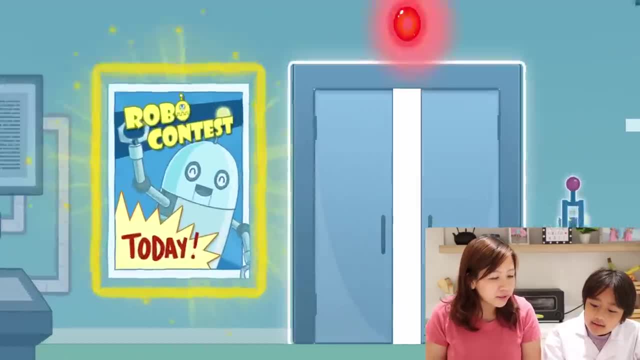 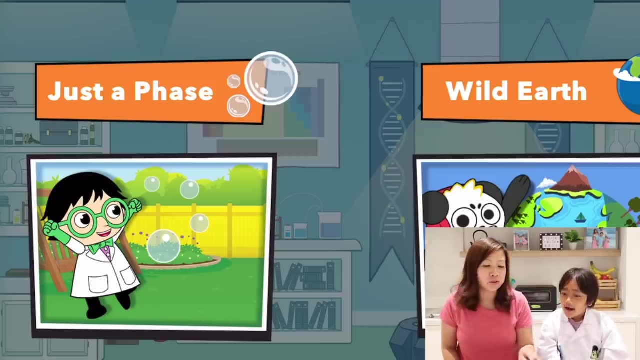 So Ryan's gonna click Ryan Then when you click on the door to get into the lab, Yeah, So in Ryan's lab there's so many different videos to choose from and learn about. Joseph Faze Wild Earth test it build it. 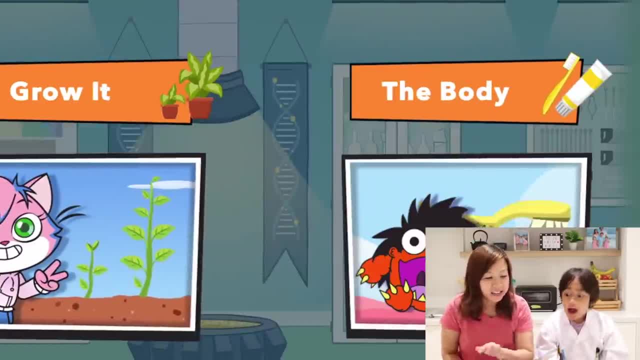 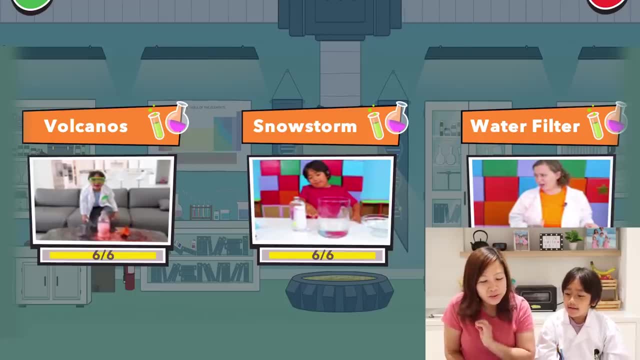 animals grow it and the body. I'm thinking today. I'm feeling it more like a Wild Earth day. What about you? Yeah, Okay. so in Wild Earth there's so many different videos too. I'm thinking water filter. 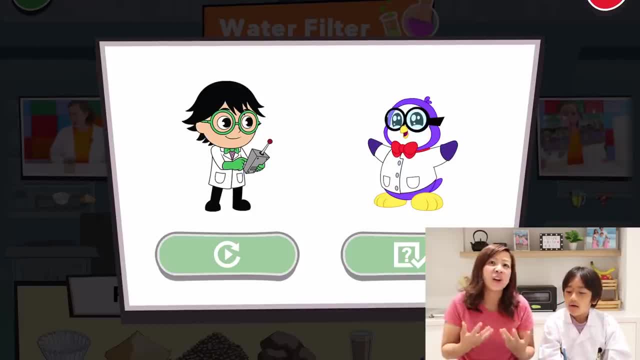 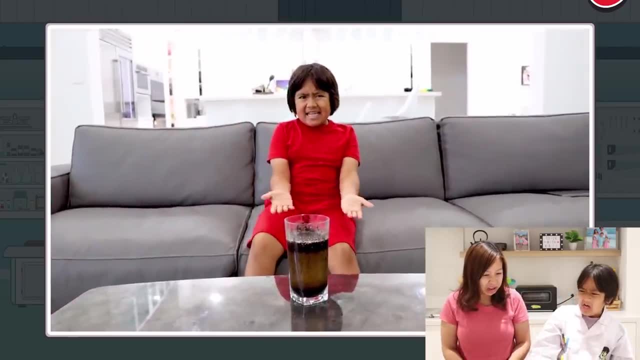 Right, Hmm, What would you do if your water is dirty or dirt? So Peck is gonna show us: Hey, Ryan, Ooh, look at that dirty water. Yeah, So Peck is gonna design a water filter. 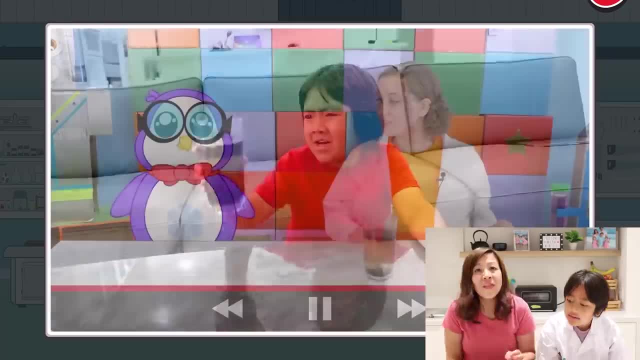 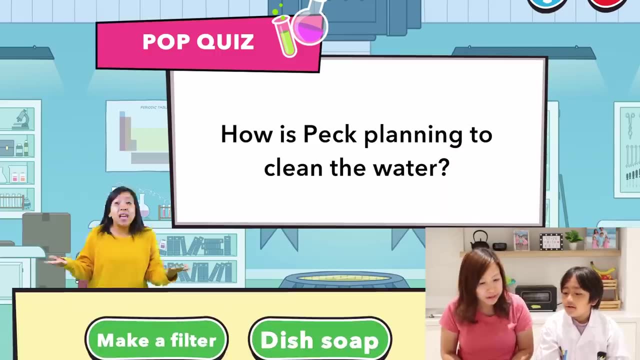 See if we can filter out that dirty water. Ooh, okay, Ugh. Then, after you finish a video, you can test your knowledge with the quiz, And it's okay, if you get it wrong, You just try again. So, Ryan, how is Peck planning to clean the water? 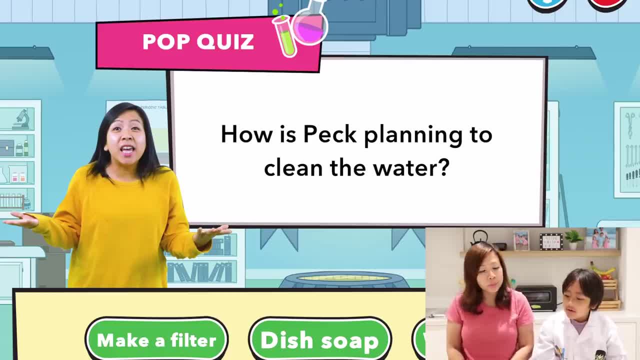 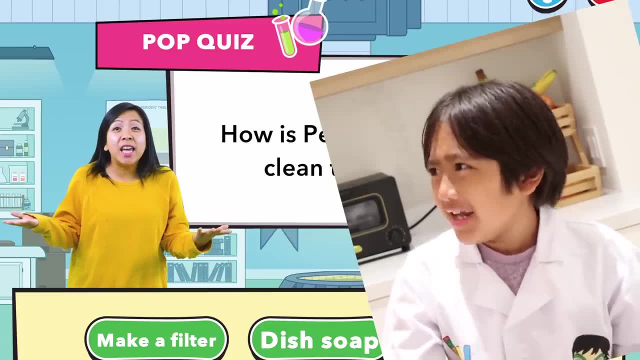 He's going to A make a filter using dish soap or warm it up. Obviously, making a filter, You do warm up dirty stuff. I don't think it's gonna do anything. Yeah, Let's see if Ryan got it correct. 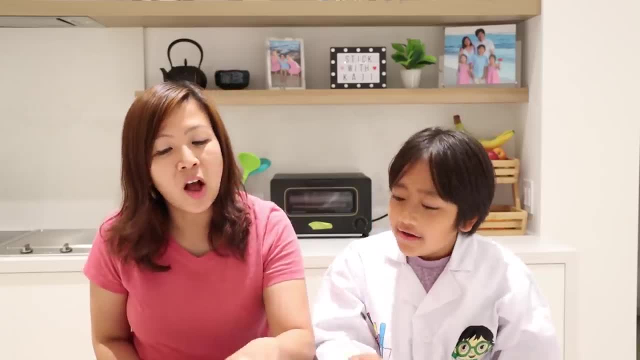 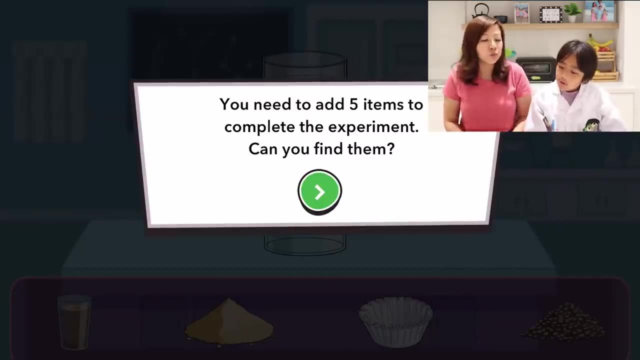 Yeah, I got it correct. Then, after you finish watching all of the videos, you can play the experiment. Okay, You can do your own virtual water filter experiment in the lab. Okay, So what's one thing you need to do? 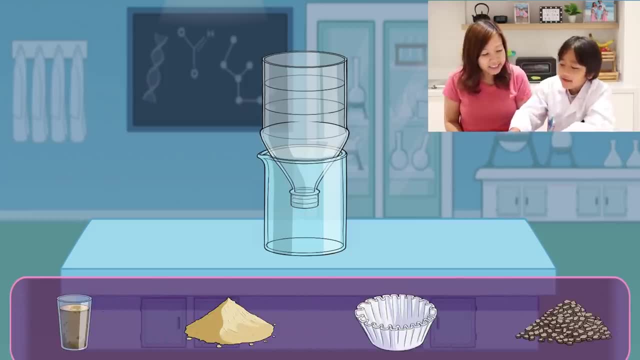 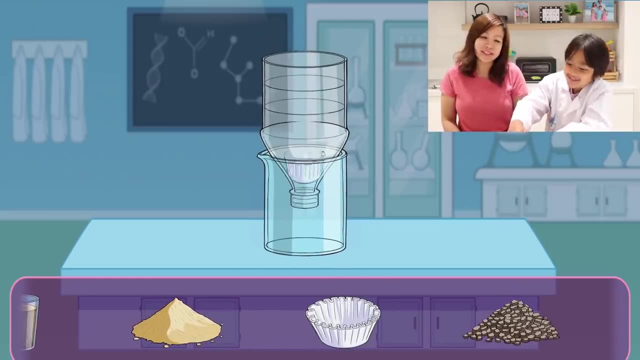 if you want to make your own water filter. Hmm, Maybe you should put this: The coffee filter Good idea Because it has a filter in it. That's right, Exactly what Peck did: Mm-hmm, And then. 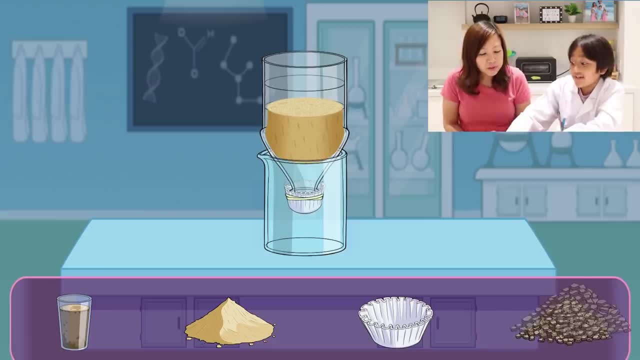 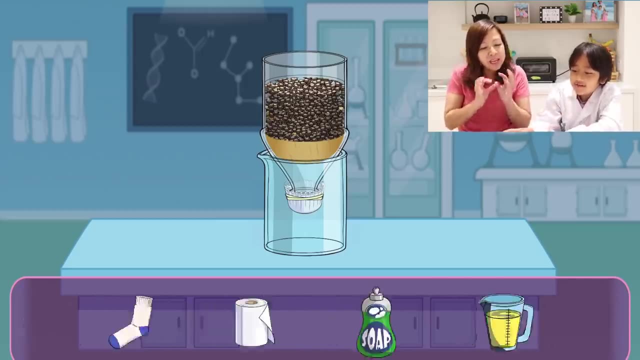 And then you should add some sand. That's a lot of sand with some gravel, Mm-hmm. So So it goes from something very, very fine like sand, something medium like a gravel. And what do you think we should use next on top? 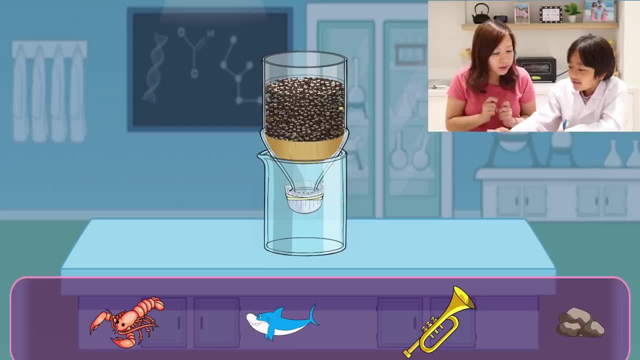 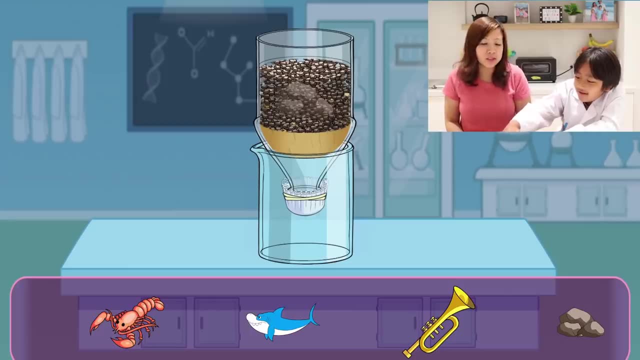 to filter out the dirt, Dirty water. I think Crab The rock circle is doing this. Oh okay, That's a lobster anyways. Oh yeah, That's right, Give you hints too. I think a lobster's a little bit too big. 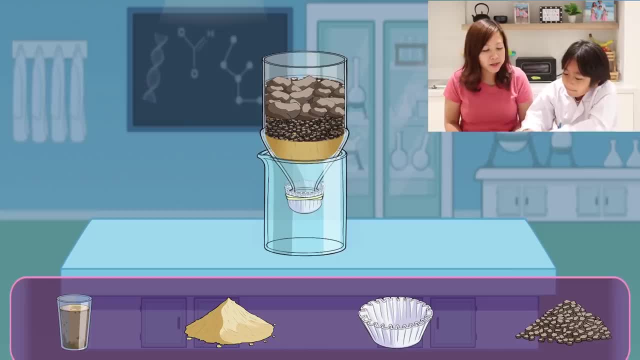 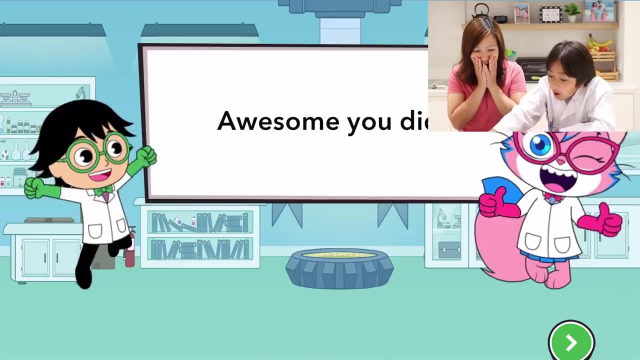 Too big? yeah, Okay. And then You think we're ready. Yeah, We need the dirty water. Okay, let's see if it's gonna work. Yay, Yay, We filter out the water. Yeah, I still shouldn't drink it though. 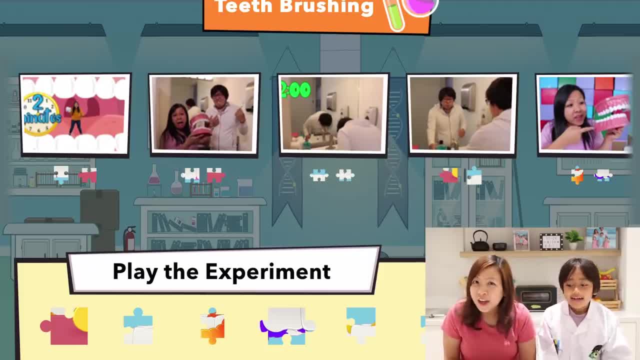 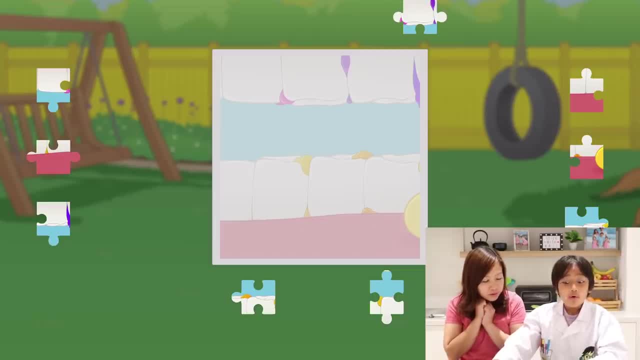 Yeah, So the other things you can do after you finish watching the videos, besides experiment, is you can do some puzzles. So what level do you wanna choose? I wanna do level one. Oh okay, Good start. I'll put this over here. 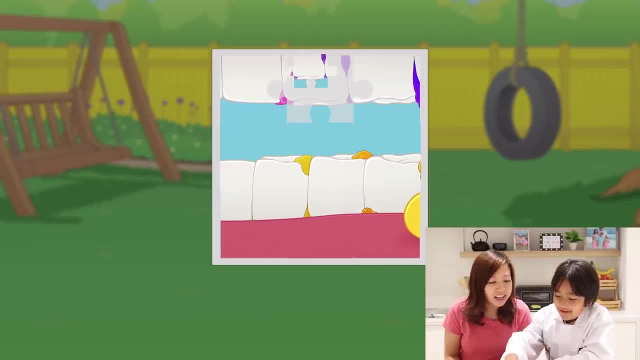 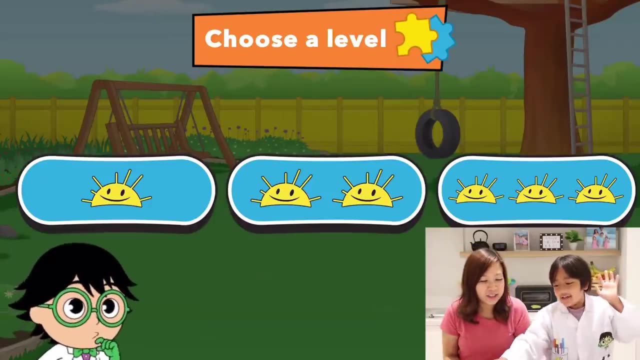 Mm-hmm. This one over here Looks like you're trying to Here, And the last one Lower: Boom, boom, boom. Yeah, You got some tea, I did it. Good, nice, You deserve three. 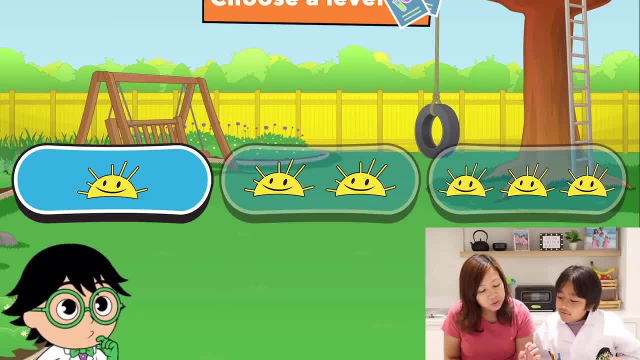 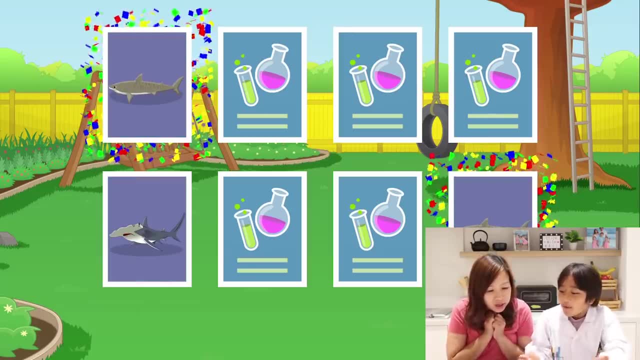 Yeah, Okay. so besides puzzles, I think you can also. I think you can also Do matching. Ooh, memory match, That's right. Ooh a shark and Oh, another shark. already You're great. Uh, another shark. 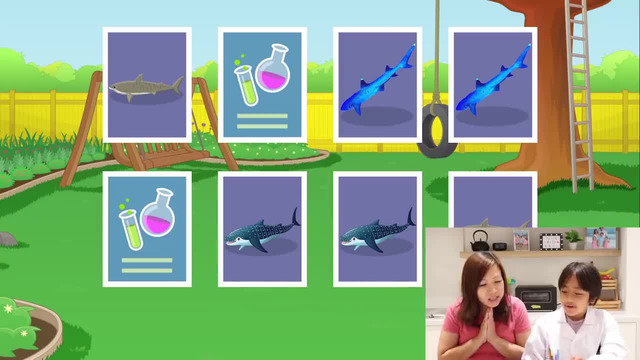 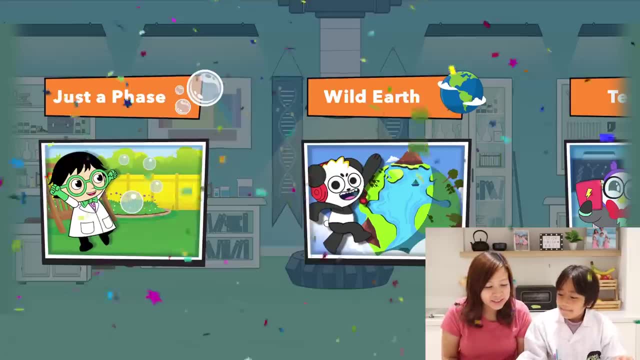 Ooh, and another shark. Another shark and another shark. Yay, Another shark and another shark. Another shark and another shark. Yay, Nice, you did it. Ooh, and the egg Is it ready? Ooh, egg. 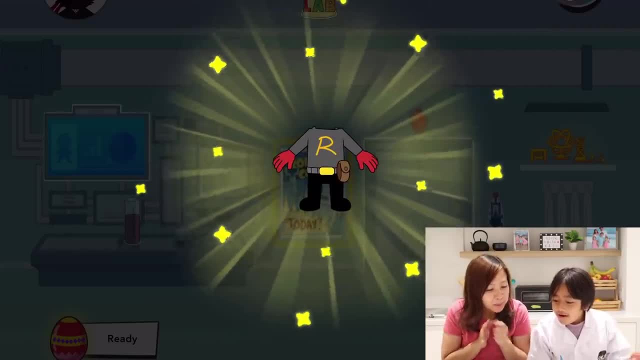 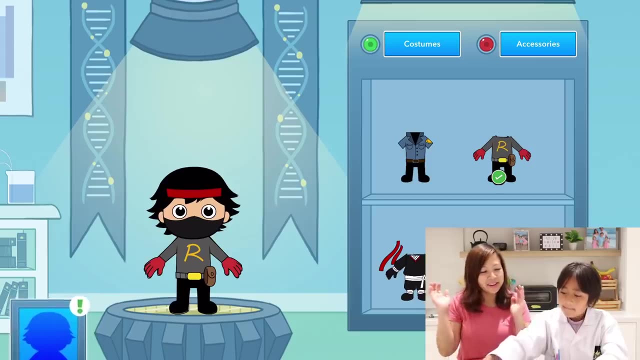 Whoa, Whoa, Whoa, Whoa. Is that a spy suit? Yeah, it's a Ryan spy suit. Nice, that means you can change outfit then. Yeah, There it is Ryan in the spy suit, Yay. 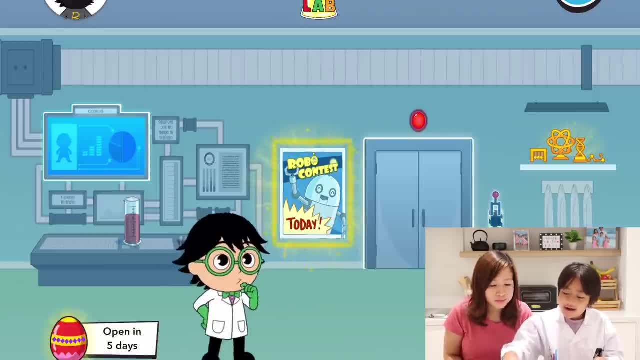 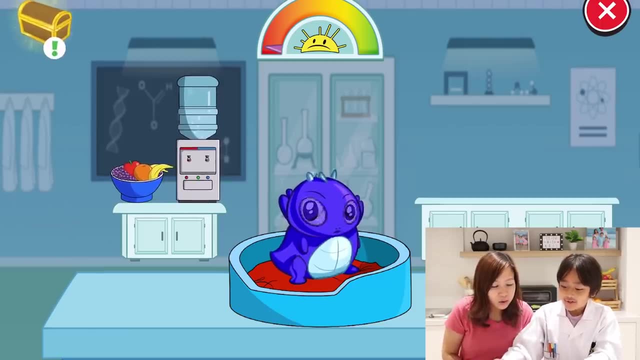 We did it. Woo-hoo, Save my changes, Of course. Yeah, Yay, and then you can also take care of your own pet dragon. Yeah, we got a new budge. Aw, Aw, Oh, it looks sleepy. 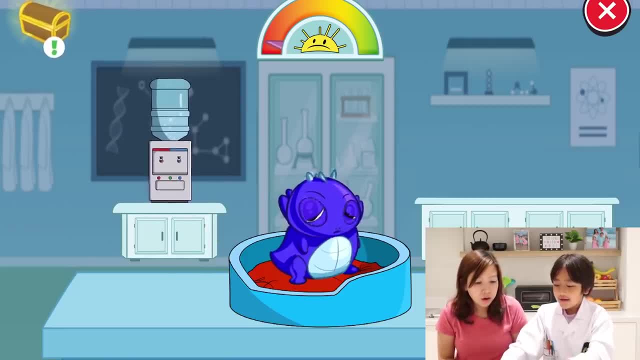 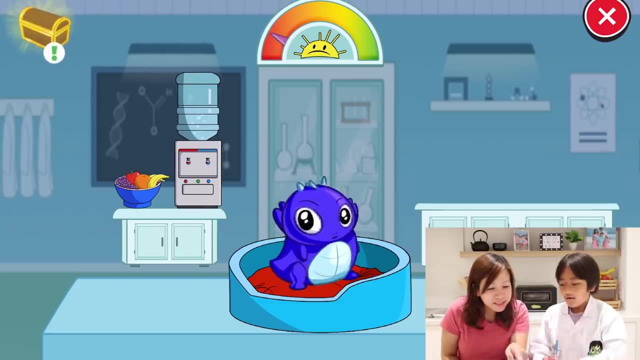 Oh, no, Maybe you should feed it food to wake it up. Yeah, Yeah, Here you go. Do you want to eat? I know, Aw, Oh, his belly is like Look, look, look, he's getting happier.